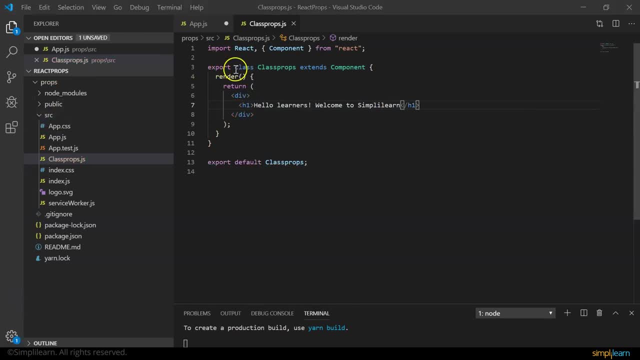 Alright, Now let me get rid of export here and import it in my appjs main component. Here I say import class-props. Alright, Now we define the class component in a render method. Let's say: alright, Now, if we go back to the browser, you see: hello learners, welcome to Simply Learn. 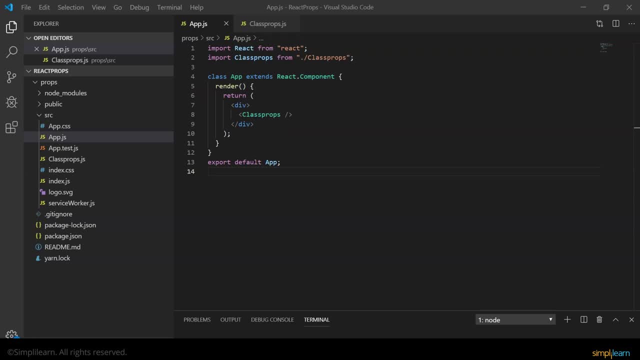 Today we want to individually welcome every student. Instead of retyping the message for everybody, we can pass their names as props. Now let's see how to do that. Now we pass the name as a property from the main component, that is, appjs to the child component, and render this onto the browser. 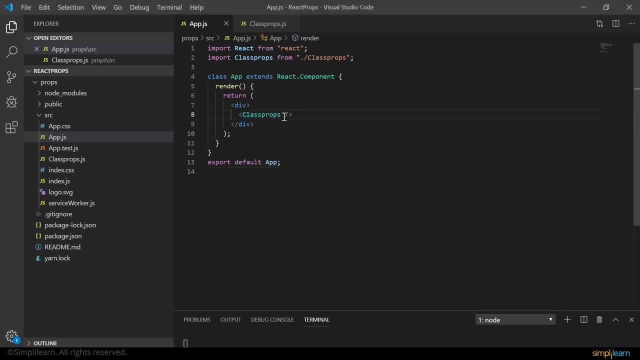 So let's do that. So here, while I'm defining my child component, I say name, I save it. In my child component, instead of learners, I say I use the keyword thispropsname, Let me save it. 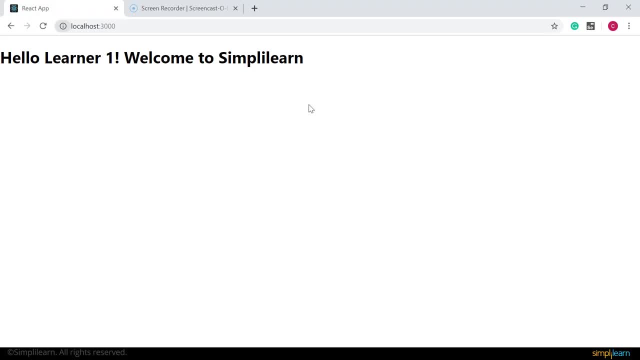 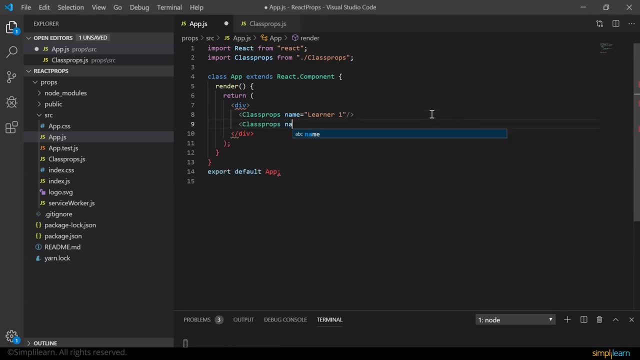 And if you look at the browser, we'll have hello, learner 1,. welcome to Simply Learn. Now let's go ahead and welcome learner 2 and learner 3.. So I again say: class-props name equals learner 2.. 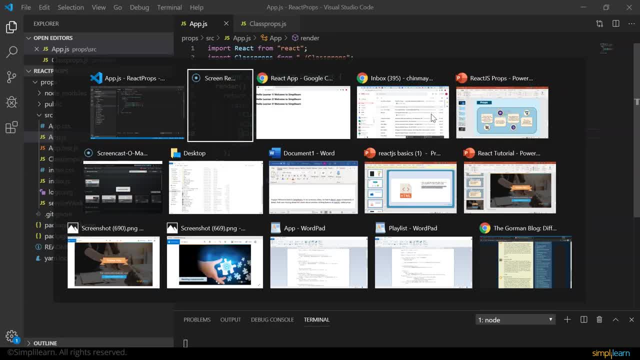 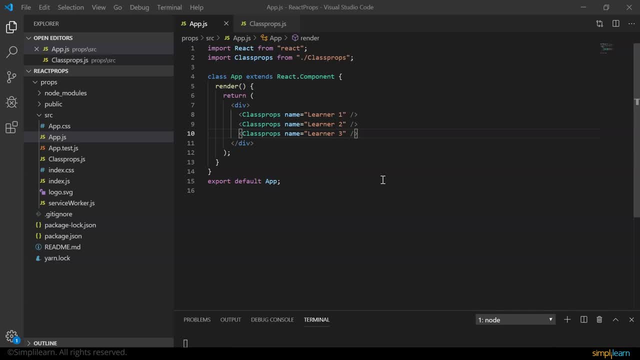 Alright. So if we save and look at the browser, we'll have all the three learners displayed on the browser. We can also pass multiple props to the child component. Now say, for example: we want to welcome the student from a particular place. 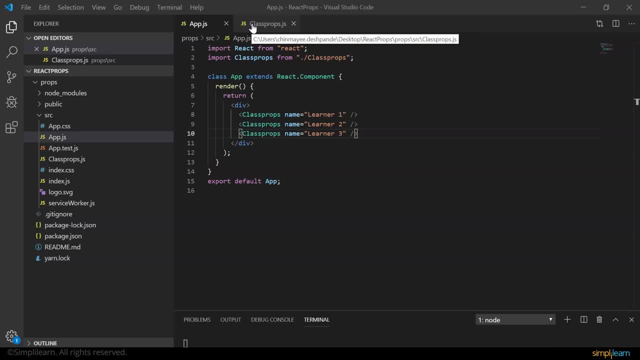 So we say: welcome, learner 1 from place x. So I can here define another property, say place, And say place. similarly, I can do it for the rest too. Say place y. Now let's go back to our class-propsjs component. 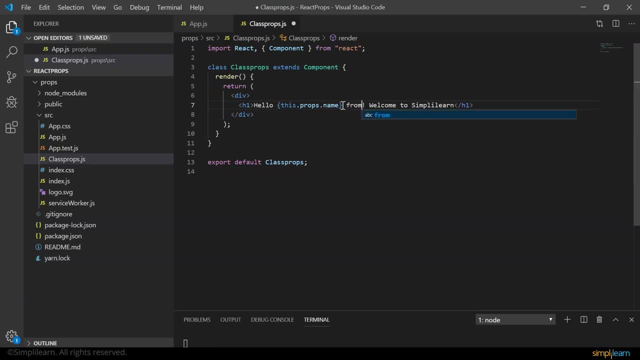 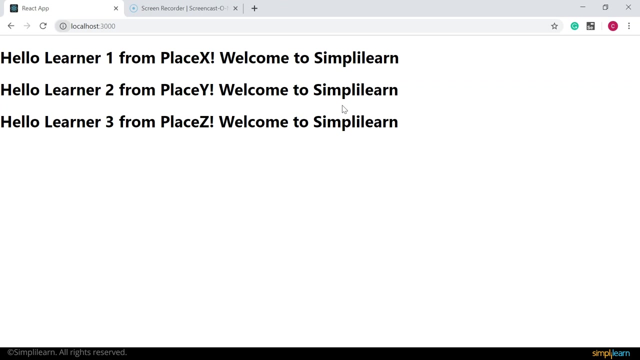 And here say hello, learner 1 from thispropsplace. Let me save it. And if you look at the browser, now we have hello learner 1 from place x, place y and place z. We can also display whatever we want between the opening and closing tags. 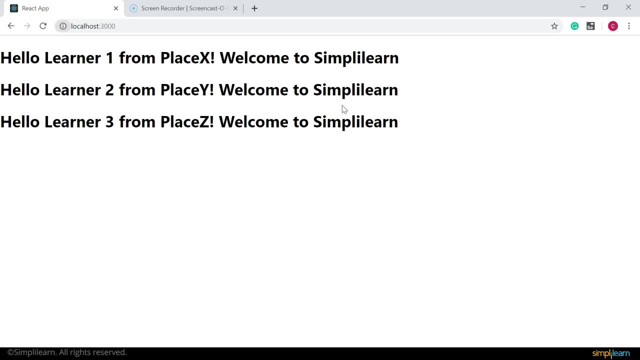 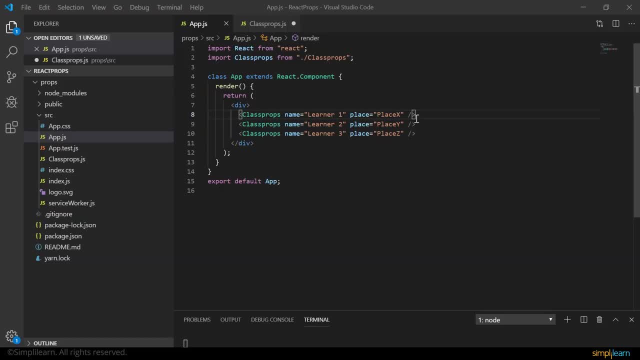 when invoking a component. Now this is facilitated using propschildren reserved keyword. Now let me explain to you how it's done with an example Here let's split the self and closing tag into an opening and a closing tag And in between them let me display a message within the paragraph tag. 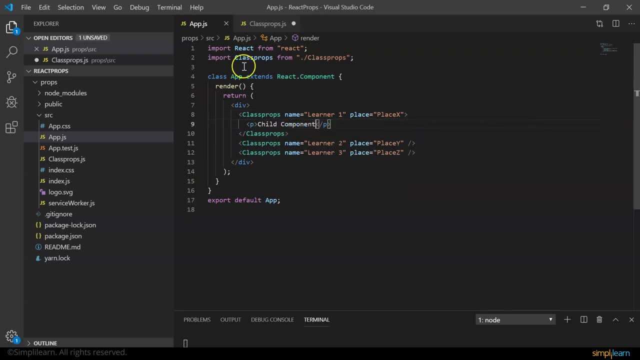 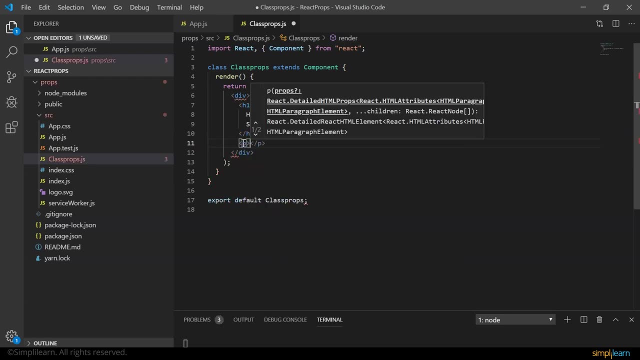 Let me save. And in my child component, after my h1 tag, let me use a paragraph tag And here let's use the reserved keyword thispropschildren. So let's save it. And now, if you look at the browser, 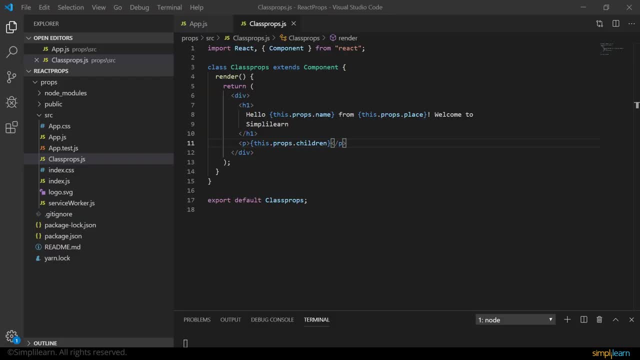 you can here see the message displayed: child component. So propschildren can be used when components do not know about their children ahead of time. This is commonly seen in components like sidebar and dialogue that represent generic boxes. So let's go ahead and create a button tag and check again. 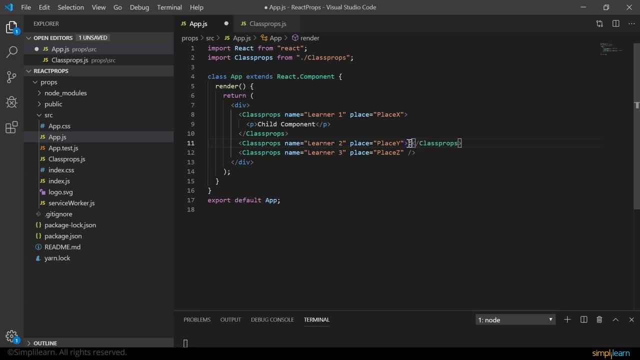 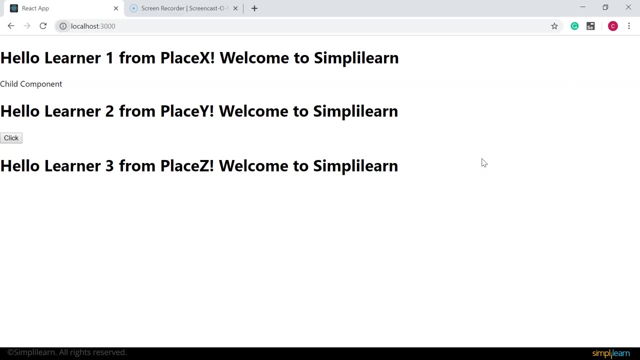 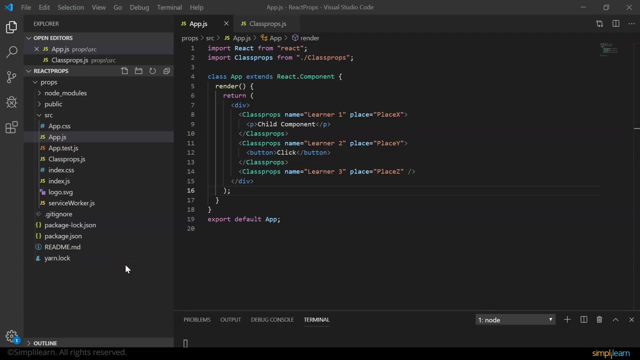 So here I'll split it and add a button tag and say: click And let's check our browser. Here we go. We get the output as expected. Alright, we saw the usage of props for class components. Similarly we can use it for functional components. 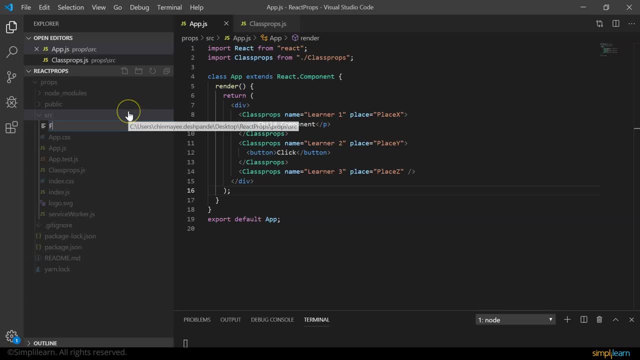 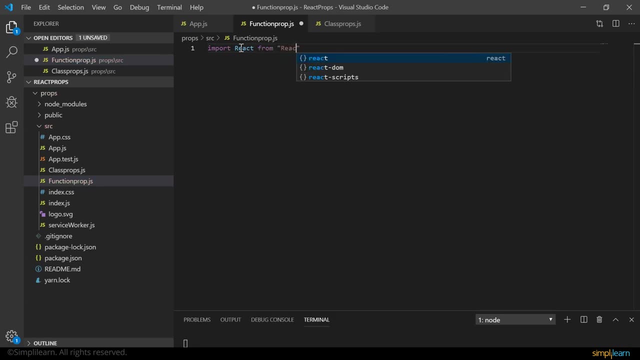 So let's go ahead and create a functional component. Let me call it propschildren. I say import, react from react, And then I say function, function props. And here I return an h3 tag. I'll say: this is functional component. 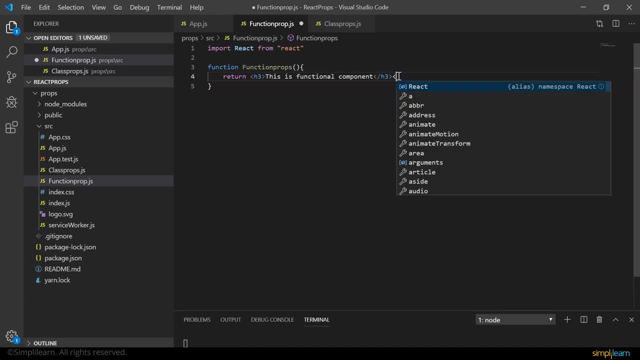 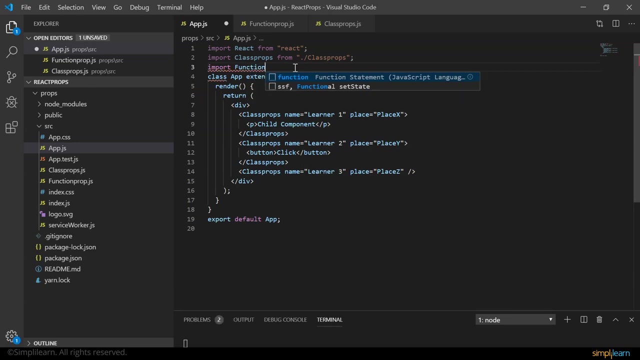 And I'll return another h3 tag saying hello learner. So let me save this. So let me save this And let's export it. Export default function props And import it in our appjs again. Import function prop from function prop.